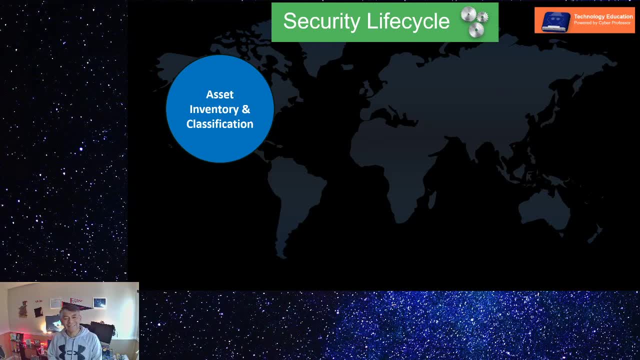 organization and finally the data that is stored and maintained by the organization. Those three components- hardware, software and data- are part of the assets that belong to a company. In the software category we identify the operating system, which is the topic of our course. So first we need to do a full 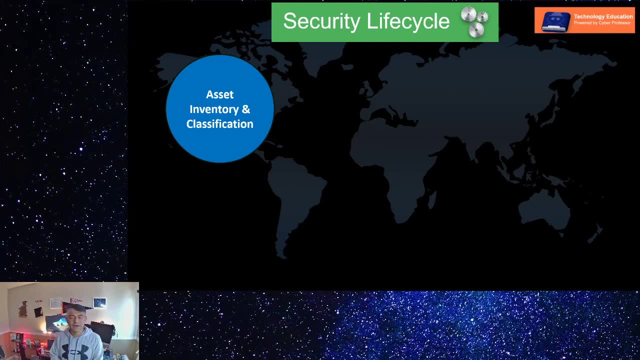 inventory of all the assets, and by that I mean identify every single hardware device, software device, including the many different flavors of operating systems that are in use in our organization and the data that is stored in our organization, And all, in this case, are integrated into the structure of Desktops of citizen. 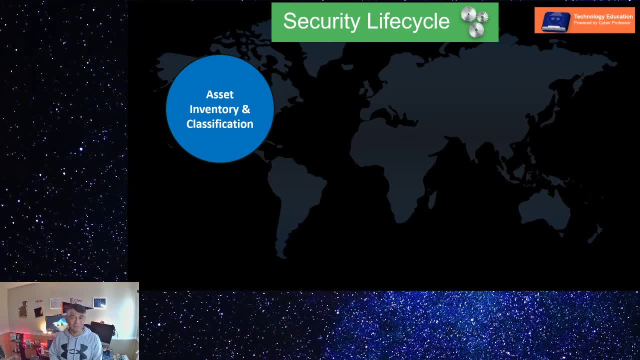 languages of a manager's name, a link to the managers analogue, and then INE digitization of all the information and put all of that information into a master database that is called the asset management database, And in this database we have a list of everything that the company owns. and then we have 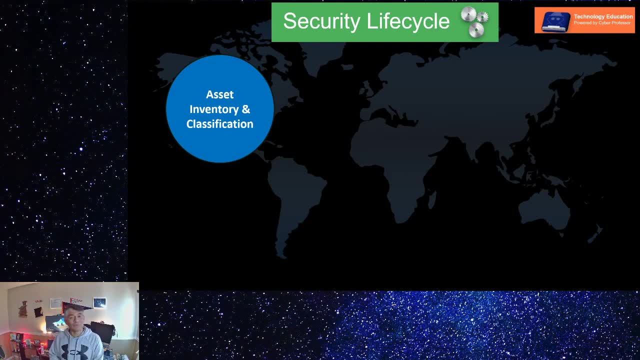 the opportunity to classinder each of those assets by the level of criticality or importance that it has for our organization. If it is an asset, the maintains-critical data- secure data, exactly data for our organization- the classification will be very high for that particular asset. If it is an asset that is not meant to store any important 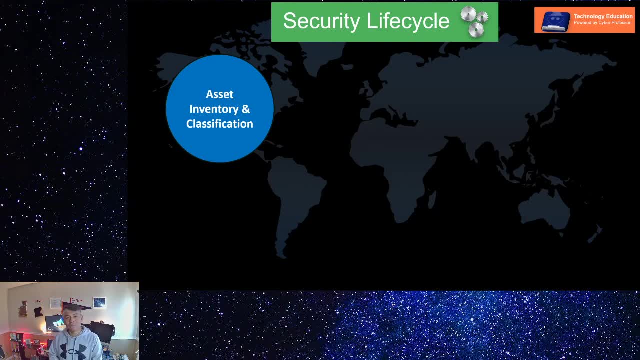 information, or critical or private or confidential information for our company, the classification for that particular asset may be very low. The next step in the lifecycle is the identification of threats. Security threats are defined as any particular external or internal agent that places the confidentiality, integrity or availability of our assets at risk. Confidentiality, integrity and 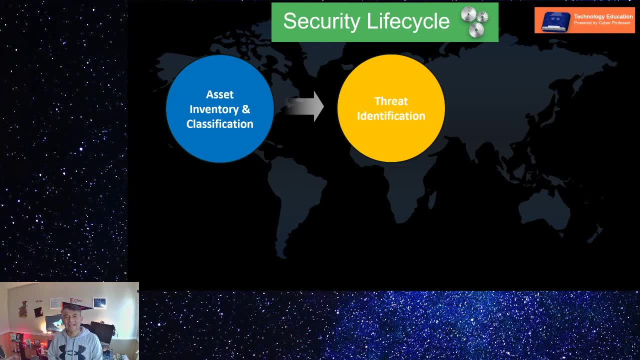 availability are the three components of the CIA. trial Security, try it- and those cannot be put at risk for any reason. otherwise our assets, including the data, will be at risk. The identification of threats includes a full inventory of any particular agent, again external or internal, that may place our assets at risk. We need to create a comprehensive 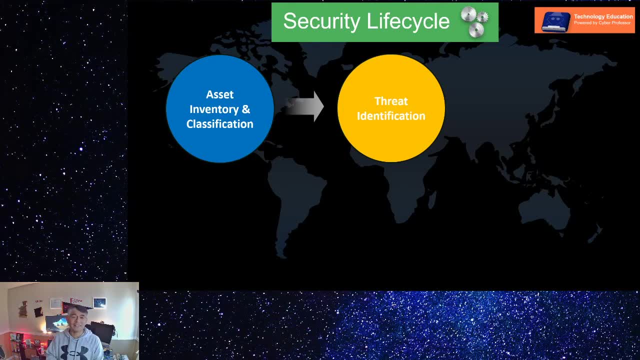 list of all threats that we believe may be identified that will put the security of our assets at risk. Examples are even natural disasters, like fire or flooding of our building, our company building, which will place all of the assets, the hardware assets, at risk within our company. Cyber attacks are also another. 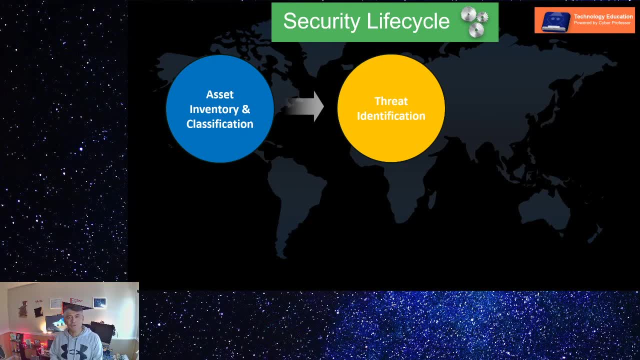 threat for our assets in the form of agents or entities external to our organization trying to break into the security of our data, our assets, our software. those are considered cyber attacks and unintentional loss of data in the form of employees that may, by mistake, place our data at risk. 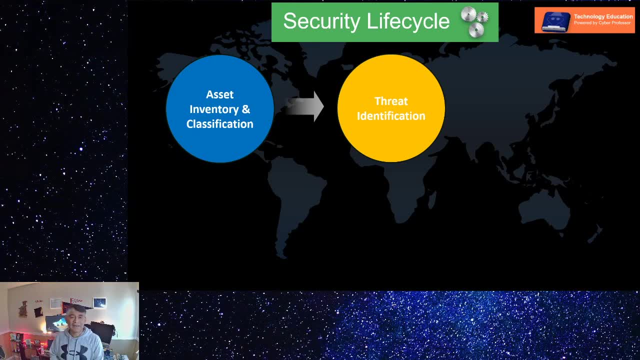 and the risk of being stolen by people that are not part of the organization. the next step in the security life cycle is the vulnerability assessment. it is a formal process that companies need to undertake in order to identify any type of vulnerability that comes with the specific assets that are part of the company. by that i mean if the company is using 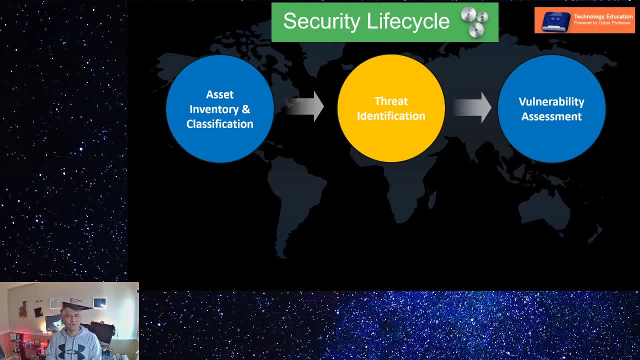 operating systems, for example, as part of the software assets that are prompt to cyber attacks, that are not properly patched because the vendor may not provide those patches in a timely manner, then the vulnerability for that particular operating system will be high. the same applies with applications- software applications that may be legacy applications, applications that were in 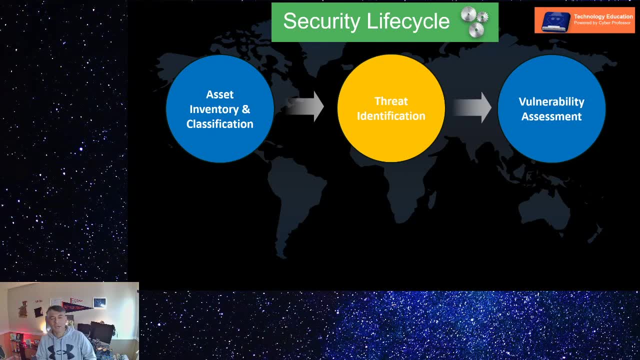 use many, many years ago, years ago- and that our company may not have been able to upgrade on a timely manner. the fact that we are using legacy applications creates a significant vulnerability- security vulnerability- for our company. a vulnerability is defined as a weakness in either hardware, software or data protection controls that we may have in our environment. 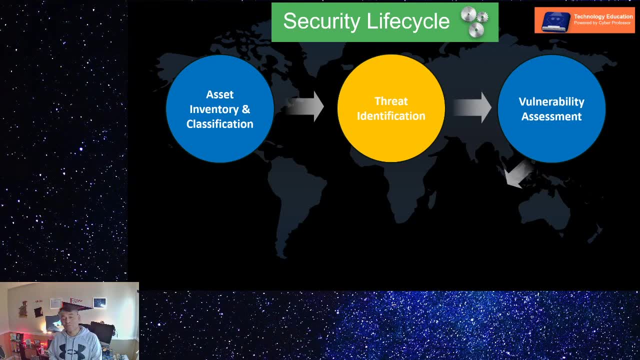 any weakness can be exploited in the form of threats that place our asset at risk. risk management is the next step of the life cycle- the security life cycle- and that involves the identification of the likelihood, meaning the probability and the impact of any threat, taking advantage of the vulnerabilities that are 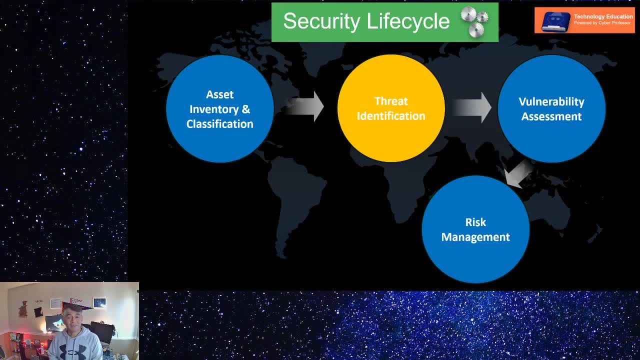 necked at our objective when we rely on take. if the risk represents there is an risks to risk management will be determined depending your vulnerability and your access to any related assets within us when ensuring the security of property and information in the entity. as the risk management process над penetration of the risk, andologie against the vulnerabilities and the likelihood of those threats. taking advantage of the vulnerabilities in our systems will be done within the company, but due to the Jack Bollinger Speaking, You gracias know I won't. the thanks for the hard work, David, Mr Knoweth, great job we have in the case of working with healthcare loan attorney and I. 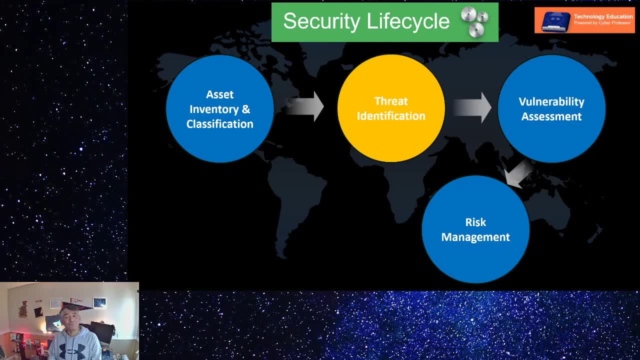 systems becoming a loss of confidentiality, integrity or availability for our assets, So that risk management process has the outcome of creating a list of risks that our companies under, in the form of high risks, medium risks and low risks that we need to protect against. 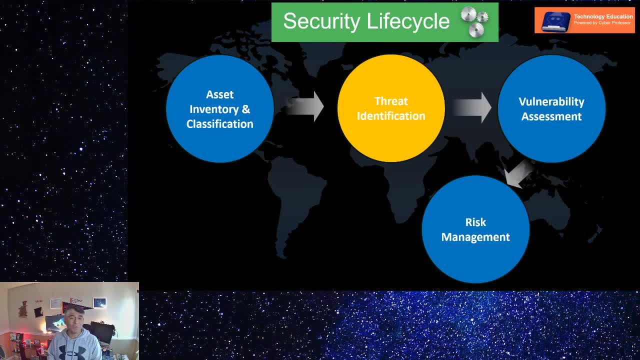 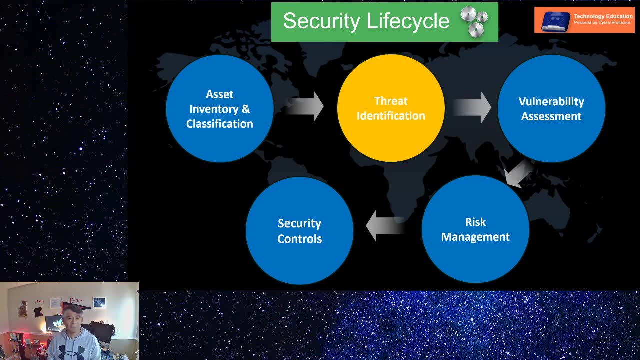 And the way to protect against those risks, in order to keep our assets secure, is by the implementation of the last step of the life cycle, which is the implementation of security controls. Security controls can be in the form of software that we purchase to protect our systems. 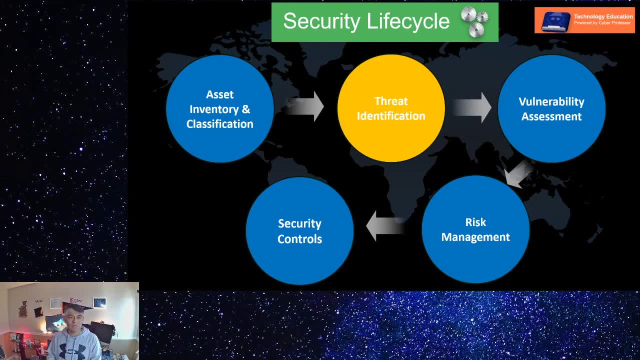 Examples of those are the antivirus software that we may place on all of our assets in our company. Security controls can also be used to protect them against viruses and malware. It can also be major equipment like firewalls that are designed to protect our systems from. 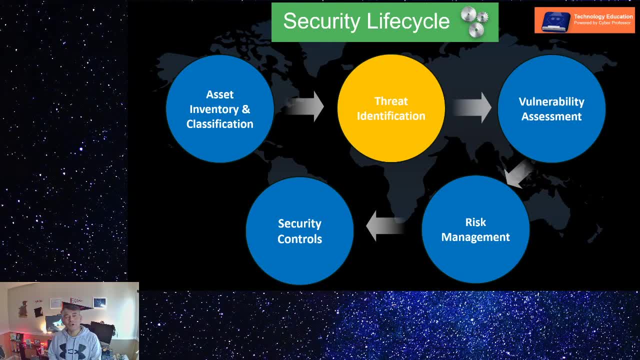 unauthorized access, Also protecting them from external agents accessing data that they are not supposed to access or sections of our environments that are highly secure. Security controls can also include the training that we offer to employees of our company, The training in the form of making sure that they do not fall to social engineering attacks. 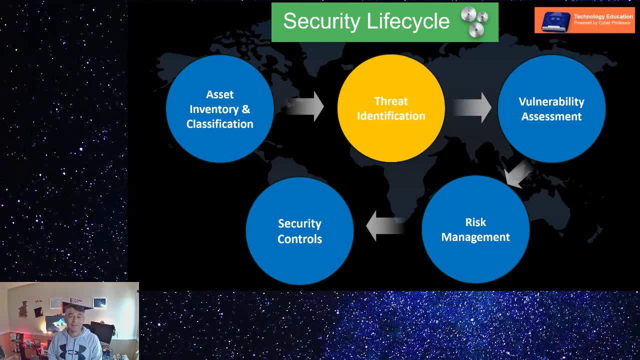 that typically come in the form of phishing emails that arrive in the company email accounts, that are prompting our employees to give up data, to give up secrets, company secrets that could open the door to cyber attacks. Training our employees against those phishing emails is also important. 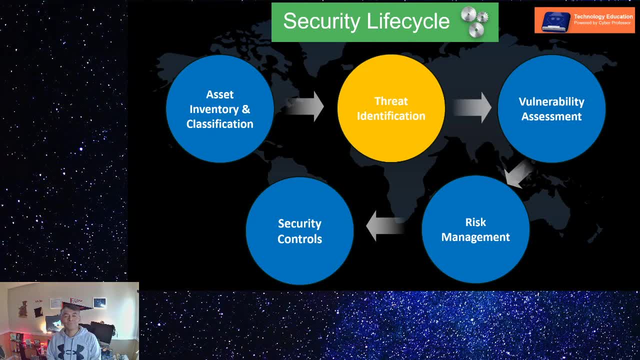 Security controls can also be used to protect our systems from unauthorized access. It's an important security control. Security controls can be software or hardware that we purchase, And by that I mean tools that we purchase. It can also be user training, And it can also be policies and procedures. 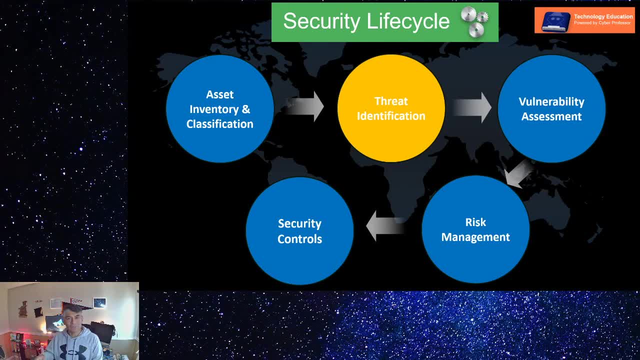 Formal written policy and procedure documents that our company develops in order to make sure that we have an organized and comprehensive process to manage any hardware, software or data that is part of our organization. so security controls are not only software and hardware that we buy. remember. security controls also include user training and it also includes 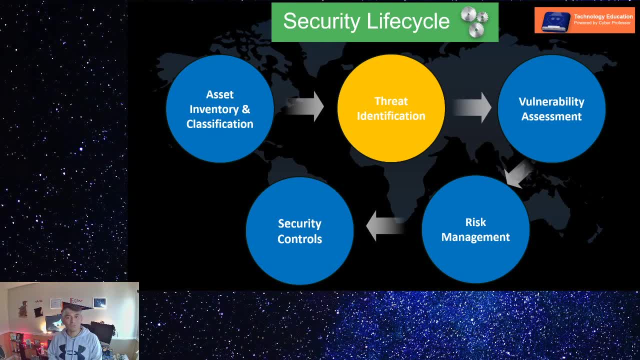 the creation of policies and procedures in written form that mandate how our company will behave. and this cycle repeats itself. the reason being: assets will change across many years and we need to continue dynamically populating the asset inventory database new assets that our company is purchasing and classifying them on a regular basis. so we continue the life cycle all over again. 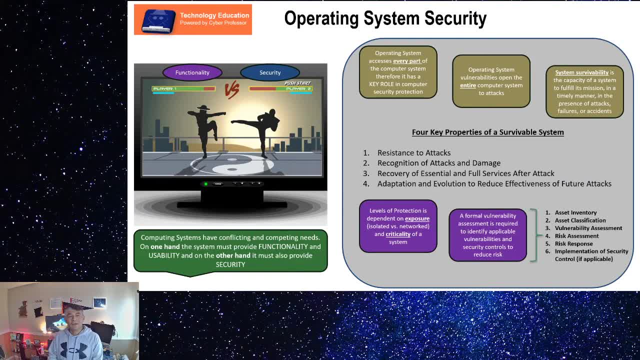 from the beginning as time goes by. now we specifically get into the security of the operating system. one of the major challenges that technology professionals have is finding a healthy balance between functionality and security. it is typically seen as the battle between functionality versus security. computing systems have conflicting and competing needs. on one hand, developers create new applications, new devices. 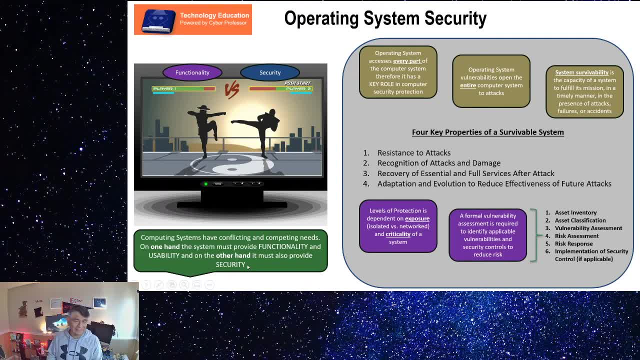 to provide functionality and usability to people in general, and that includes operating system features that are deployed by the major software vendors like Microsoft. Microsoft Windows operating system has many features that are created to enhance the functionality and usability of the operating system: shortcuts, ways of giving users the ability to do things in a faster and better way within the 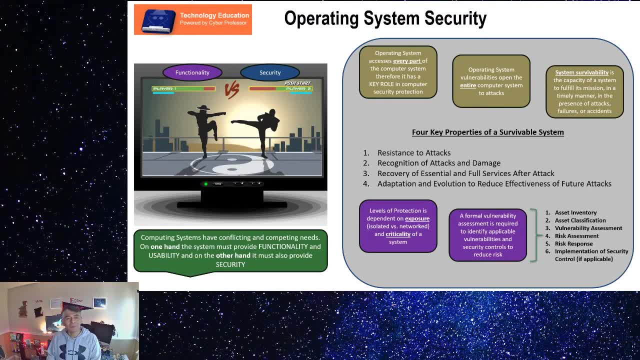 operating system within the Windows operating system is part of the effort of creating additional functionality and give that functionality to you, the user. however, many of those functionality enhancements come with severe security flaws and finding the balance between giving more functionality, making things better as far as the user experience. 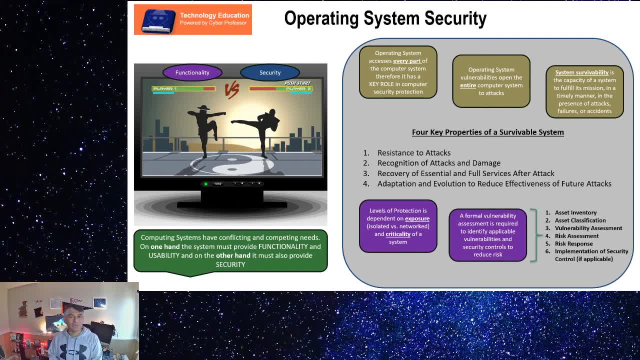 has to be. it has to take into account the security implications of that functionality that we are giving to users. so again, the takeaway is: finding the balance between functionality and security is critical for the efforts of keeping our operating system secure. operating systems are unique in who, in that they access every part of the computer system. therefore it plays 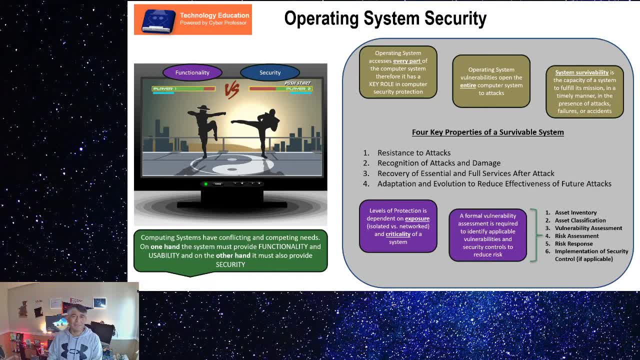 a key role in keeping computer security in place for you, the user, and for organizations as a whole. operating system vulnerabilities have the capability of opening the entire computer system to cyber attacks. another reason to take operating system security very seriously- system survey solver probability is the capacity of a. 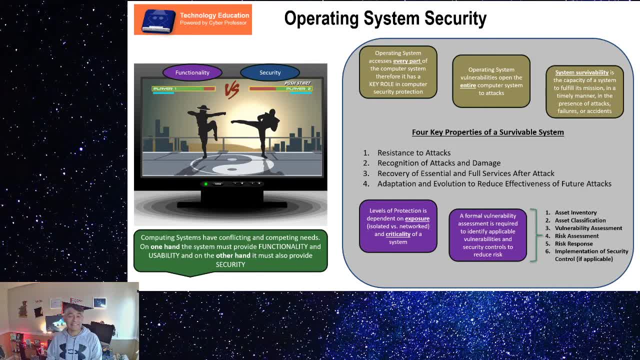 system to fulfill its mission in a timely manner in the presence of attacks, failures or accidents. there are four key properties of survivable system: the resistance to attacks, the recognition of attacks and damage. the recovery of essential and full services after an attack. and the adaptation and evolution to reduce effectiveness of future attacks. the levels of 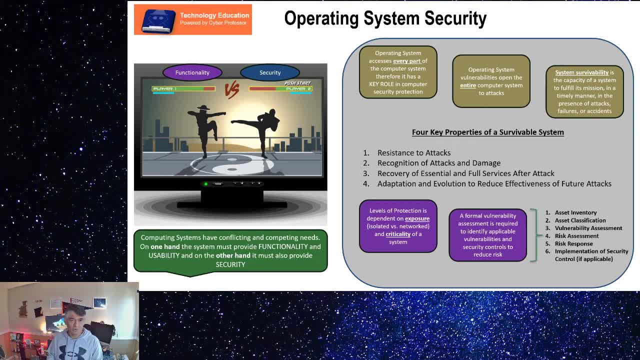 protection are dependent on the exposure of the computer system that we are trying to protect. if the computer system is isolated, a set of level of protection steps will be taken that may not be as critical and as uh high effort as systems that are exposed to the network. and also we need to take into account the 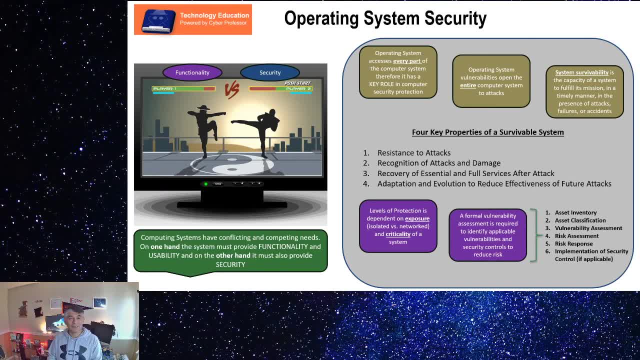 criticality of the system that we are trying to protect. on that particular step, the classification of assets, which was presented in the previous slide, is a critical component. a formal vulnerability assessment is required to identify applicable applicable vulnerabilities in security controls to reduce the risk. these are some of the steps that we discussed earlier today: the asset inventory. the asset. 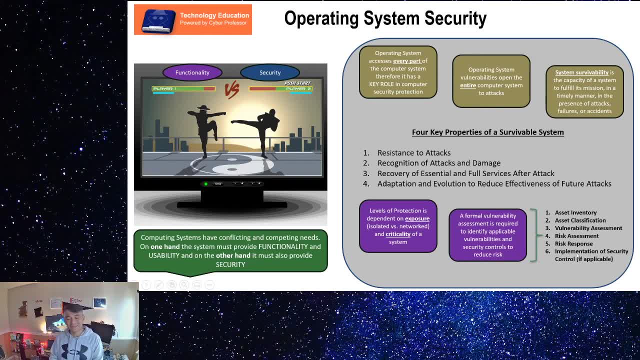 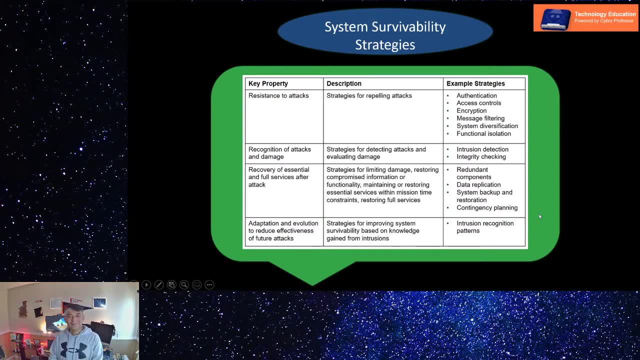 classification, the vulnerability assessment, the risk assessment that risks response and the implementation of security controls if applicable. the system's server ablility strategies are as follows, as we mentioned. the first one is the to attacks and the description for that is the strategies for repelling attacks. 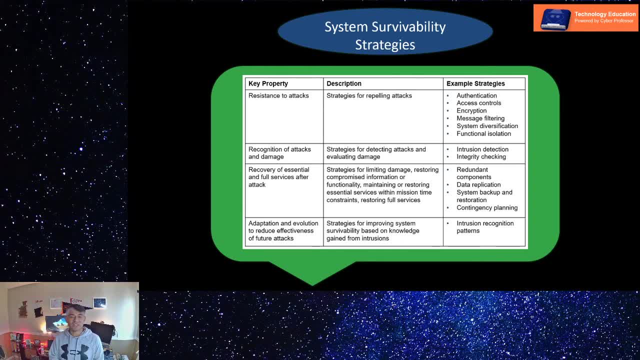 We need to make sure that we create strategies for repelling the attacks, the cyber attacks. Examples of those strategies include the authentication of users that are trying to access the different assets in our organization, including the operating system, access controls, encryption, message filtering. 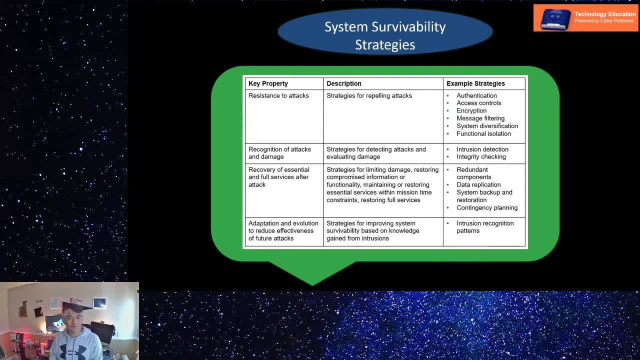 system diversification and, finally, functional isolation. The second key property of a system is the recognition of attacks and damage. Operating systems need to be capable of recognizing attacks and the damage that comes with those attacks In that form, strategies for detecting the attacks and. 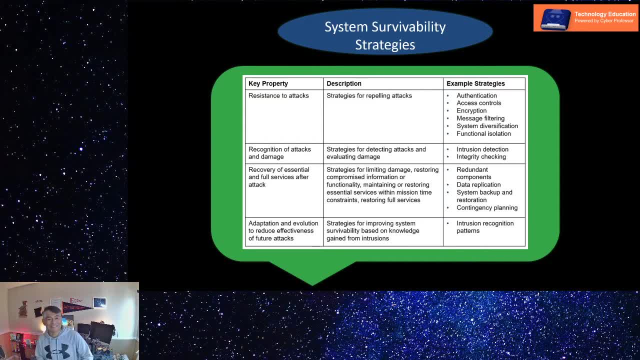 evaluating the damage must be created as part of a review. Strategies to implement that particular property include the intrusion detection and the integrity checking. Another key property is the recovery of essential and full services after an attack, and the description of that particular property involves the strategies for limiting damage. 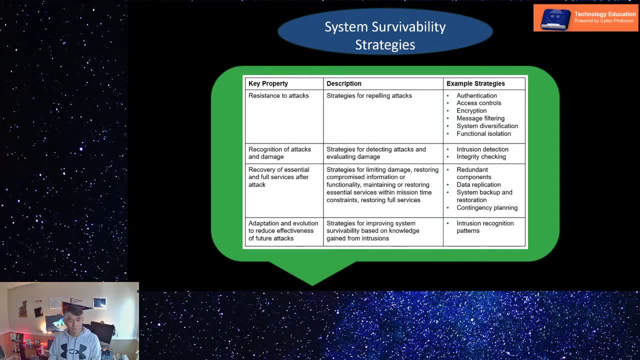 restoring compromised information and the use of the information to improve the functionality. One of the key core Imaginative benzene cryo-cal 근데 tune mechanism: Scorpio for communication or functionality, maintaining or restoring essential services within mission time constraints and restoring full services. Examples of that particular key property include data backups, system backups, backups of the operating system itself. redundant components- meaning placing devices that are of high criticality for our organization based on data. Laura Baker, Fulger and beyond. 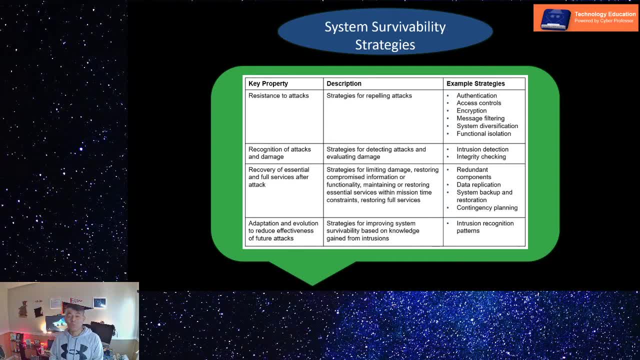 different locations so we can counteract any natural disaster that may impact our organization. if a location in our company is subject to flooding, then we need to make sure that we create a redundant copy of that particular system with its operating system in a different location that is not subject to. 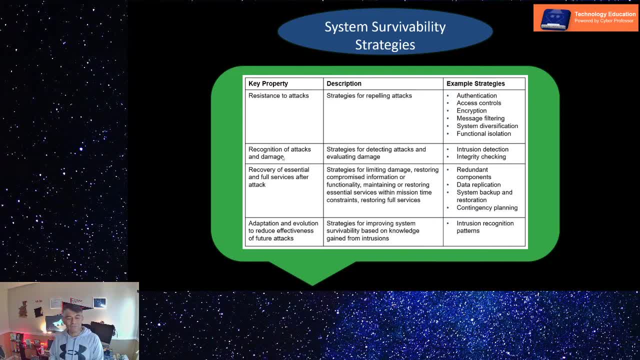 flooding. Adaptation and evolution to reduce effectiveness of future attacks is the last property that we are discussing and that involves the strategies for improving systems survivability based on knowledge gained from intrusions. Intrusion recognition patterns is an example of that strategy becoming part of our regular activities in our company. 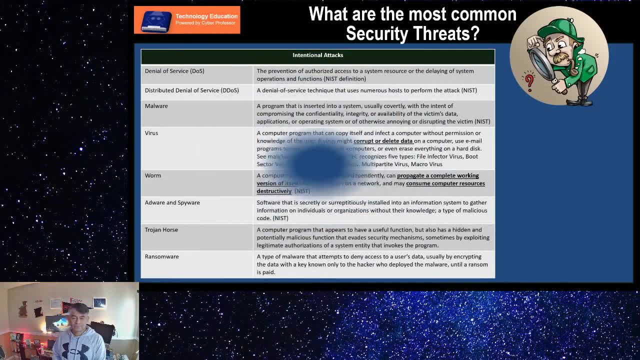 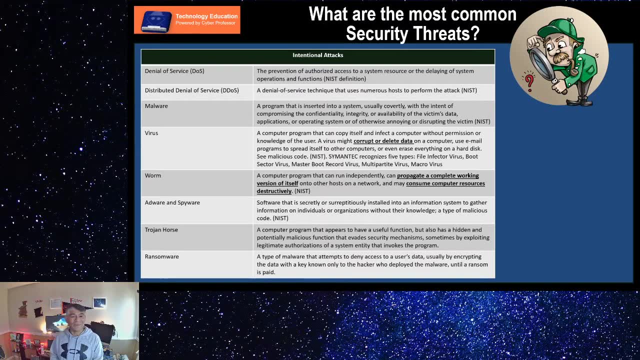 We need to ask what are the most common security threats? There are intentional attacks in the form of denial of service or DOS, which involves the prevention of authorized access to a system resource or the delaying of system operations and functions, and that is based on the NIST definition. NIST is 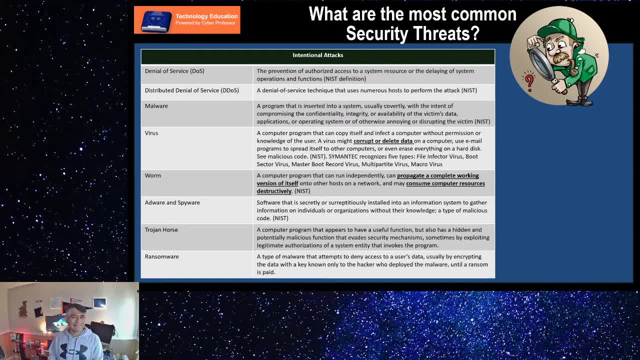 the organization that provides many different standards in the form of documents that are published for the use of private and public companies in the topics of cyber security. Distributed denial of service or DTOS, which is a denial of service technique that uses numerous hosts to perform the attack. 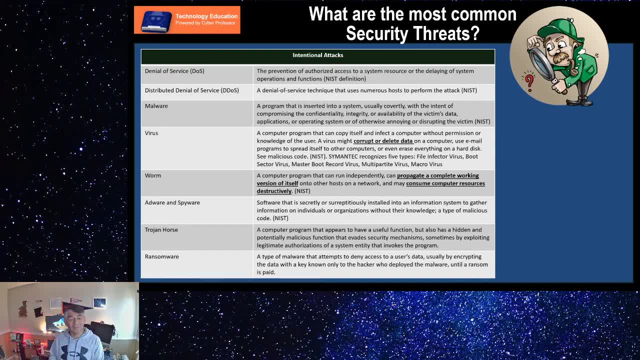 Malware is another example of an intention, intentional attack. Malware is a program that is inserted into a system, usually covertly, with the intent of compromising the confidentiality, integrity or availability of the victim's data, applications or operating system, or of otherwise annoying or disrupting the victim. 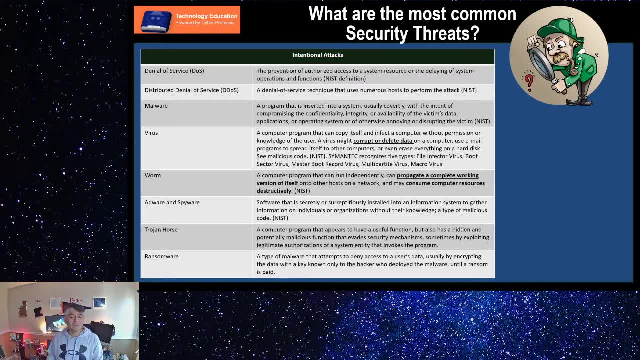 Virus, A computer program that can cap itself and infect a computer without permission or knowledge of the user. It is important to know that a virus might corrupt or delete data on a computer, use email programs to spread itself to other computers or even erase everything on a hard disk. 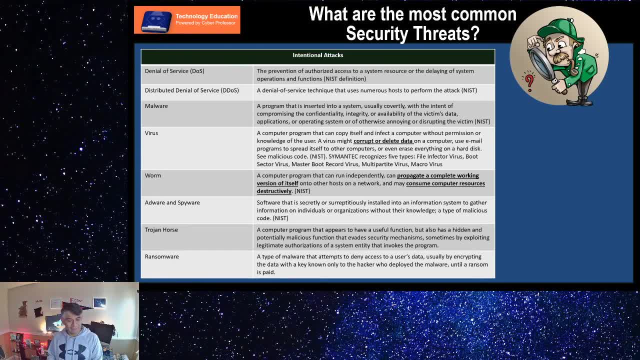 Worm, A computer program that can run independently, can propagate within a complete working version of itself into other systems on your network, Invent And may also consume computer resources destructively. Adware and spyware Software that is secretly or surreptitiously installed into an information system to gather information on individuals or organizations without their knowledge. 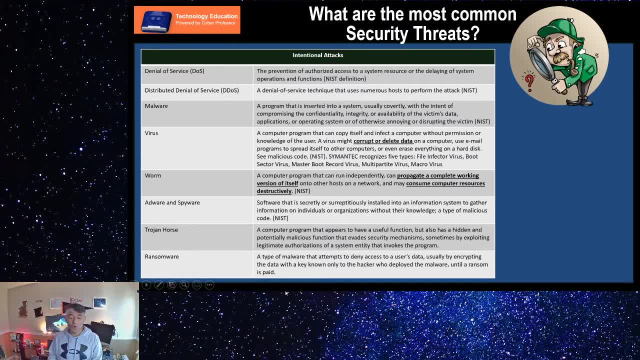 A type of malicious code Trojan horse, A computer program that appears to have a unique useful function, but also has a hidden and potentially malicious function that evades security mechanisms, sometimes by exploiting legitimate authorizations of a system entity that invokes the program. 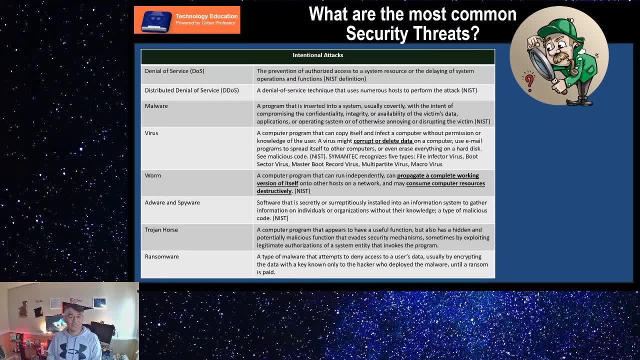 And finally, another major example of an intentional attack is ransomware, which is defined as a type of malware that attempts to deny access to a user's data, Usually by encrypting the data with a key known only to the attacker who deployed the malware, until the company that owns the asset pays the ransom. 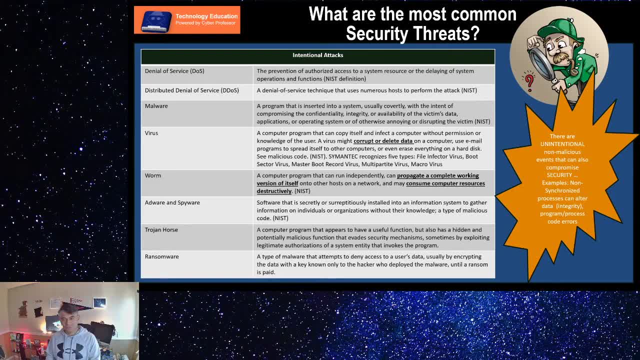 Finally, there are unintentional, non-malicious events that can also compromise the security of the operating system. Examples include Non-synchronized processes that can alter the security of the operating system. Examples include Non-synchronized processes that can alter the security of the operating system. 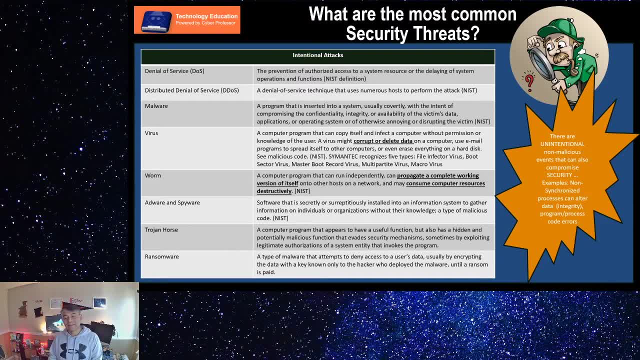 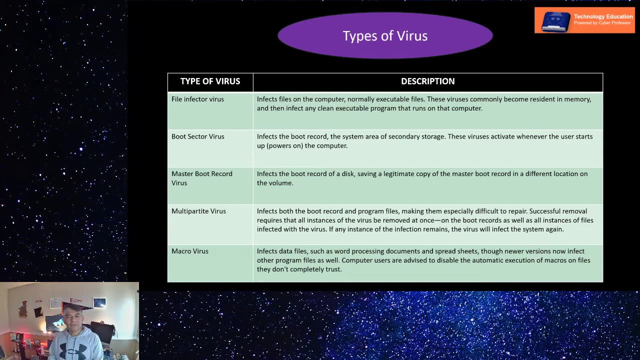 data, the integrity of your asset and the program or process code errors that are typically part of any development process in the operating system applications. here we are going to define some of the most important types of viruses that you may have to deal with in your activities. as far as protecting, 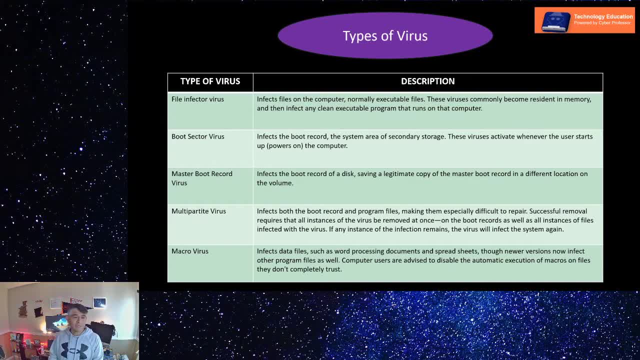 the operating system security. the first type of virus that we are going to discuss is the file infector virus. this virus attacks the files, infects the files that reside on a computer, normally executable files. these viruses commonly become resident in memory and then interact, infect any clean executable. 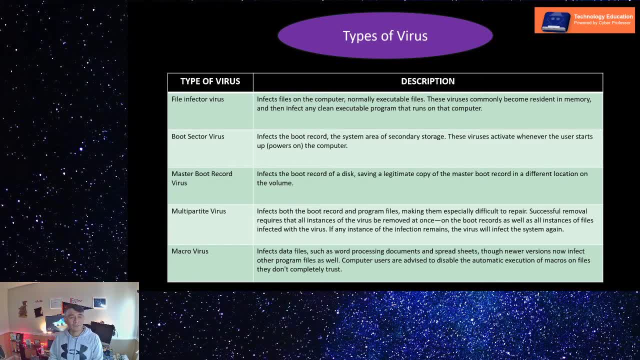 program that runs on that particular computer. another type of virus is the file infector virus. this virus is the file infector virus, that is, is the boot sector virus. it infects the boot record, the system area of secondary storage hard drive. these viruses activate whenever the user. 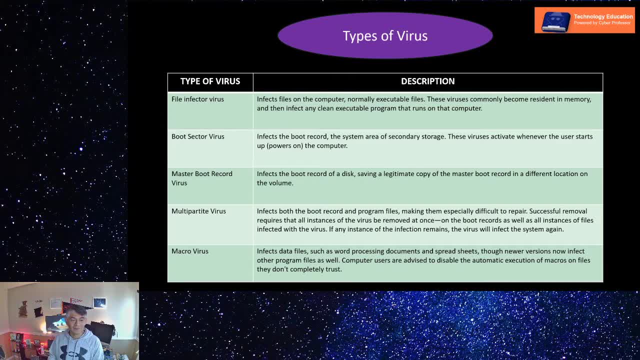 powers on the computer system. master boot record virus is another example or type of virus. it infects the boot record of a disk, saving a legitimate copy of the master boot record in a different location of the volume. multi-partite virus infects both the boot record and program files, making them especially difficult to repair. 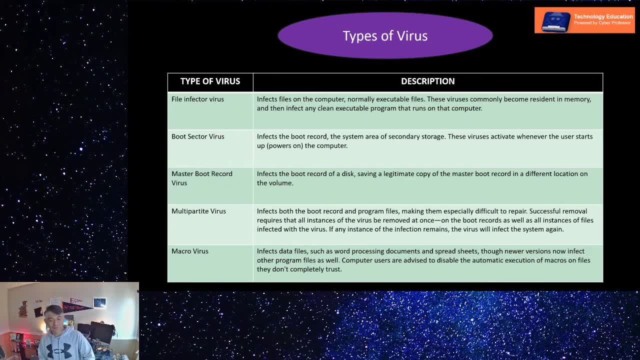 successful removal requires that all instances of the virus be removed at once on the boot records, as well as all instances of files infected with the virus. if any instance remains infected, the virus will become infected. after using the Zakir virus. we will check if any brings clean. afterinte, もulty, apartheid virus, artists and viruses can be found online application likemaq and verificationstyle. 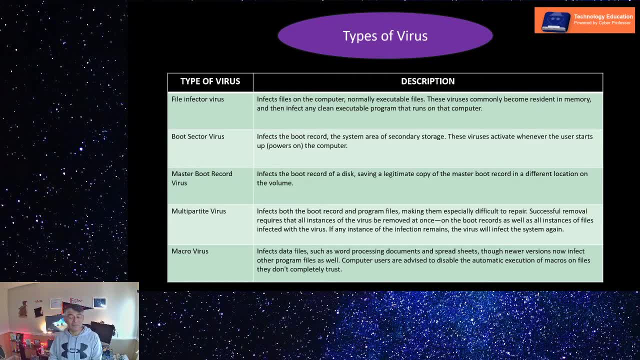 virus. we will check if any I brings and filters is weeks from several weeks remaining, if any I brings and filters is not crowded. prevent становs virus contain all instances of files infected on the boot records, as well as all instances of files infected with the virus in case most of the virus is self protected. 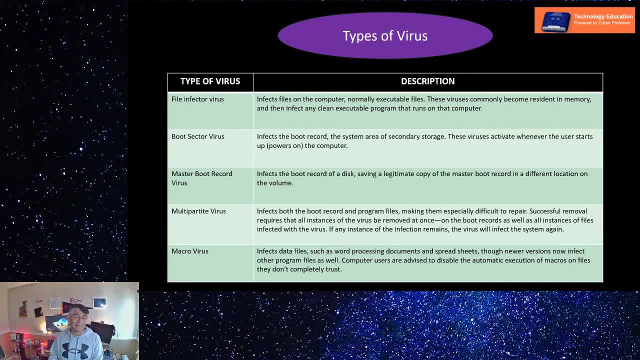 from all instances of the virus. the virus will leave the path for himself, the one from your device to any other device. the virus will continue to negatively impact the computer system. Finally, macrovirus: It infects data files such as Word processing documents and spreadsheets. 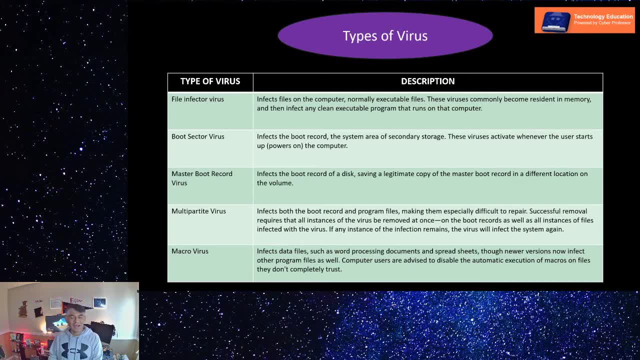 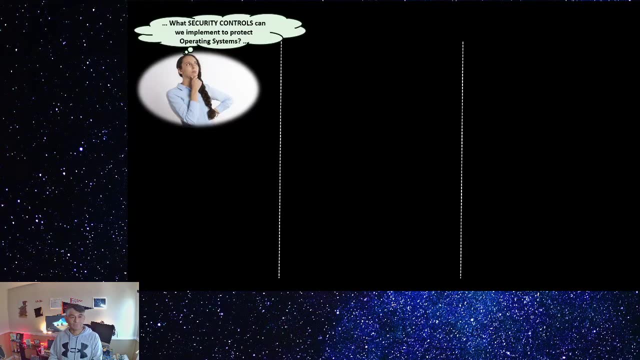 Microsoft Excel, Microsoft Word are typical applications subject to this type of viruses. Computer users are advised to disable the automatic execution of macros on files they don't completely trust. So the next question that you may ask yourself is: what security controls can you implement to protect operating systems? Those include 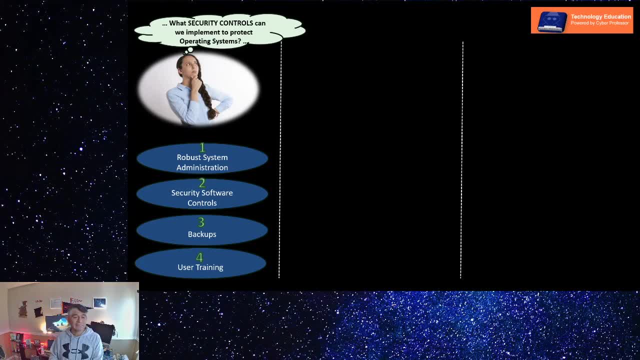 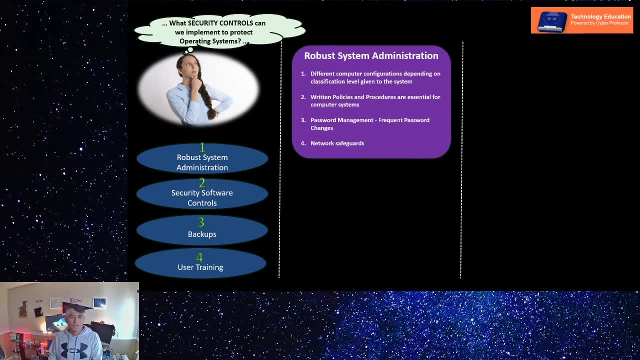 robust system administration, security, software controls, backups and, finally, user training. For robust system administration, we have the following activities: Creation of different computer configurations depending on the classification level given to that particular asset or system. The creation of written policies and procedures to protect. 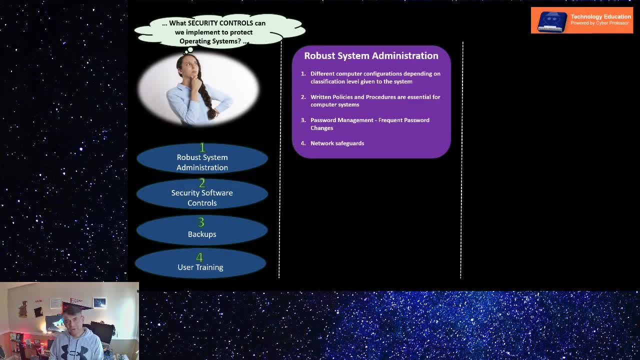 computer systems in the form of what software highly critical systems will receive and will be approved to be installed on them, And that particular list will be maintained and will be written in a policy or procedure that is part of the company's documentation. Password management includes the frequent changes of passwords for all the users that 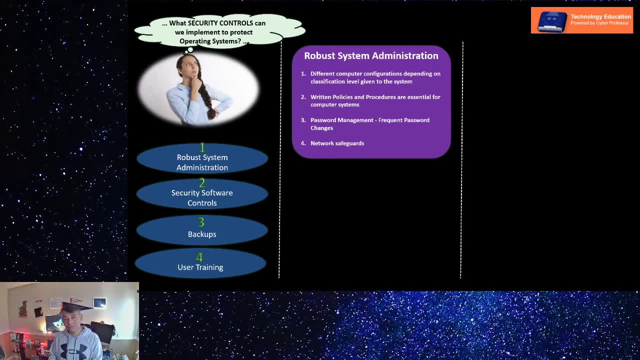 are accessing the different computer systems, in order to protect and secure operating systems on those systems. Finally, Network safeguards: the creation of steps to the access to the network environment for our organization. At the end of the day, those safeguards will be the ones protecting the operating system. 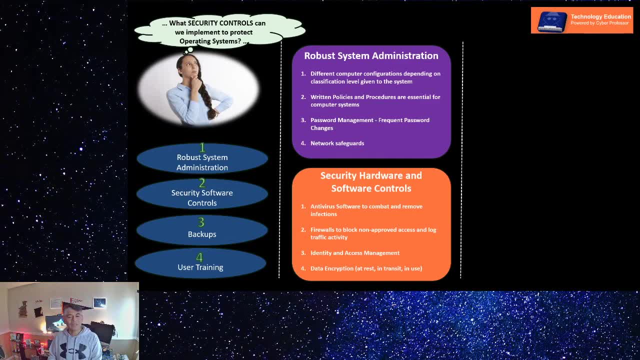 residing on our assets. Security hardware and software controls. Antivirus software to combat and remove infections, Installed on every single device that has the capability of receiving those viruses or malware. Firewalls to block non-approved access and to facilitate the logging of traffic activity within. 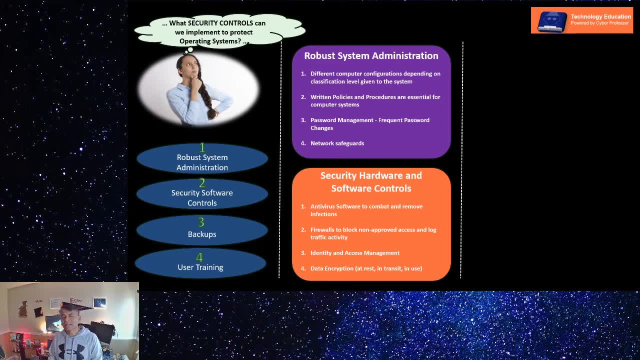 our network Identity and access management: The creation of a sound and secure identity and access management program within our organization that will allow us to access our network. Credentials to be given to employees and users based on the needs- the functional needs- they have to access company data. Data encryption, A form of 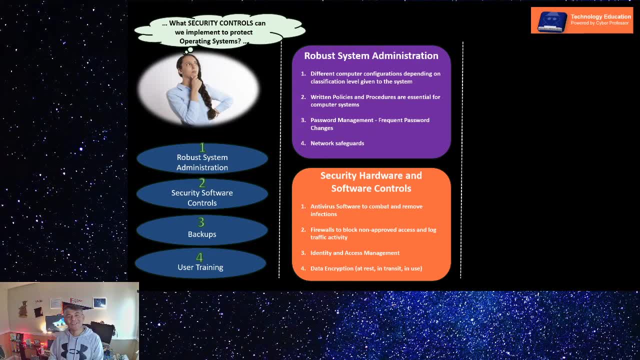 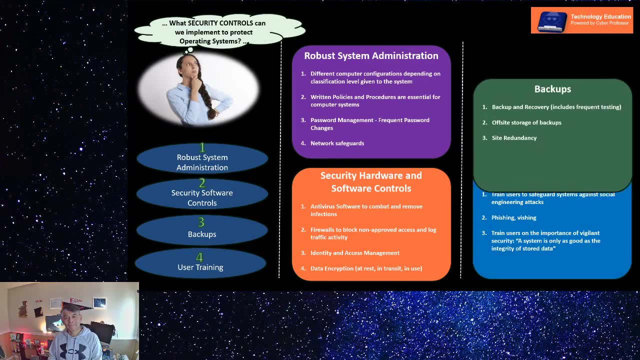 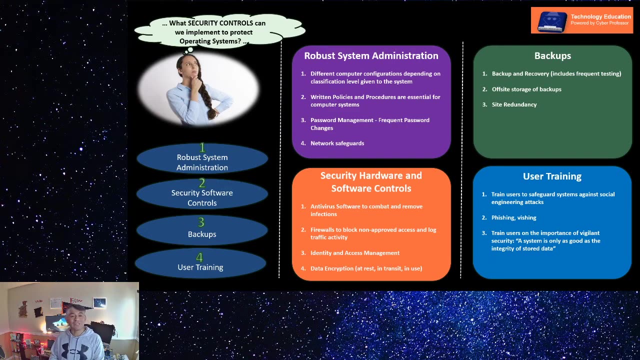 process and software to be used to encrypt data at rest, in use or in transit Backups. Backup and recovery includes the frequent testing of the backups, the backup jobs and the recovery or restore jobs that are part of the software that is used to backup our data. The use of off-site storage for the backups, either.